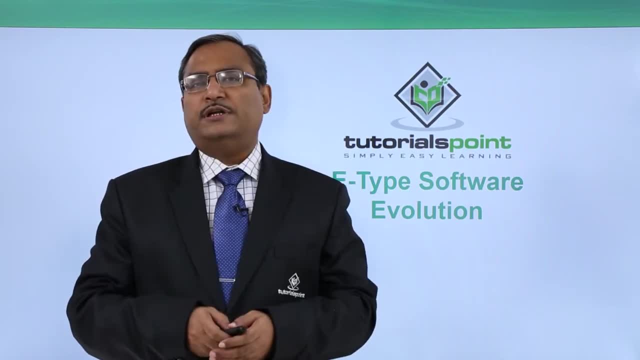 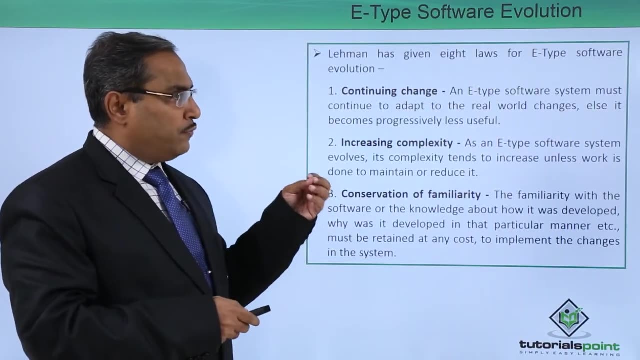 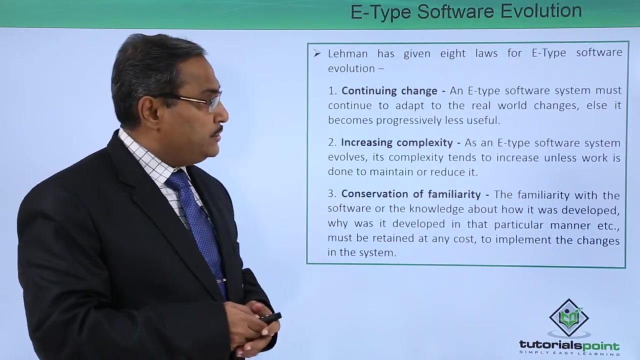 in this particular session, we are discussing E-type software evolution. So now let us go for the further detailing. Lehman has eight laws for this E-type software evolution. So what are the eight laws? are there The first one: continuing change and 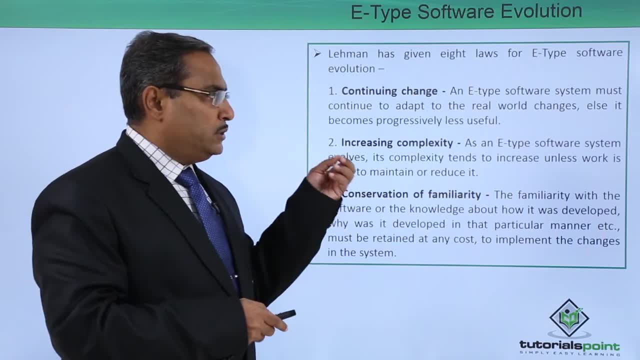 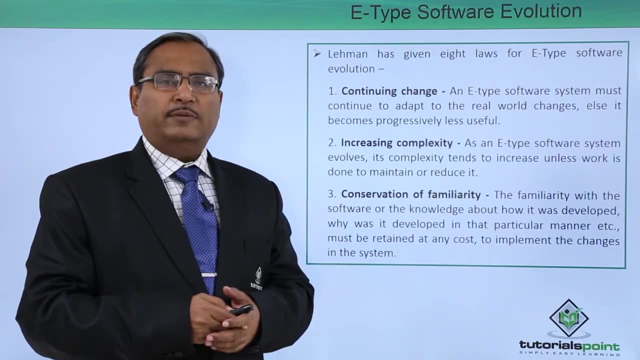 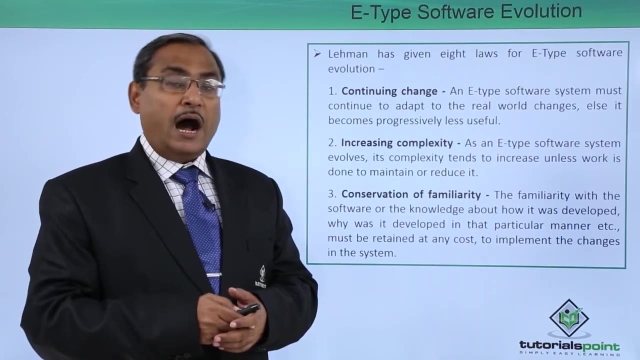 E-type software system must continue to adapt to the real world changes, Otherwise it becomes progressively less useful. Change requests will be coming from the client, from the users, and those change requests has to be, they are to be implemented in the software. Otherwise, in the long run the software will become useless. 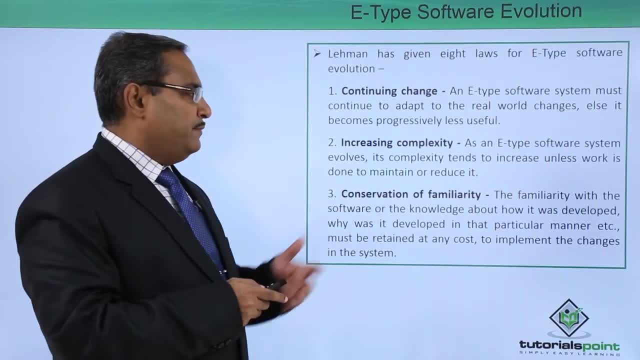 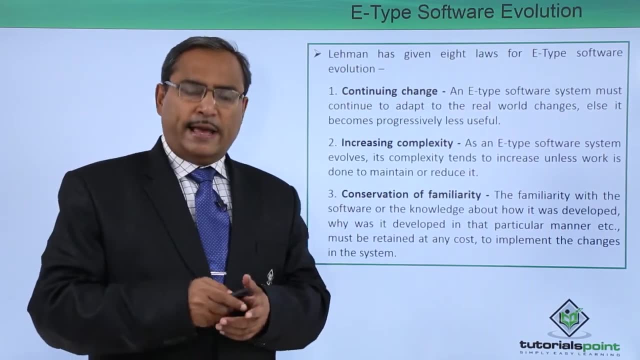 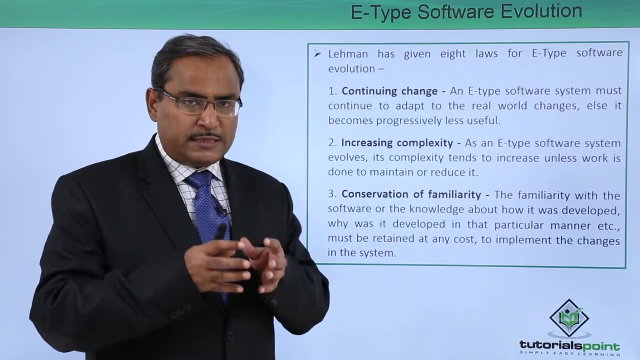 Increasing complexity. As an E-type software system evolves, its complexity tends to increase unless work is done to maintain or reduce it. The complexity of a software will increase. So we should have to do some preventive measures. Some actions are to be taken to maintain it and to reduce it. 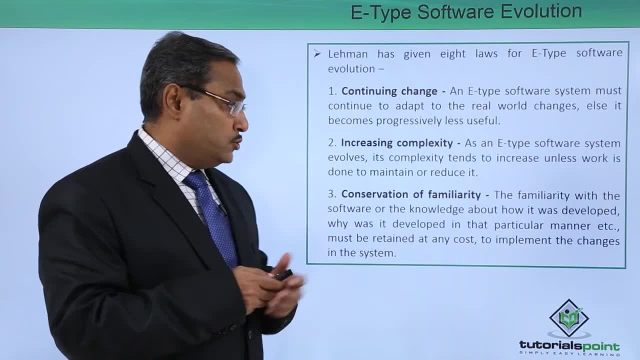 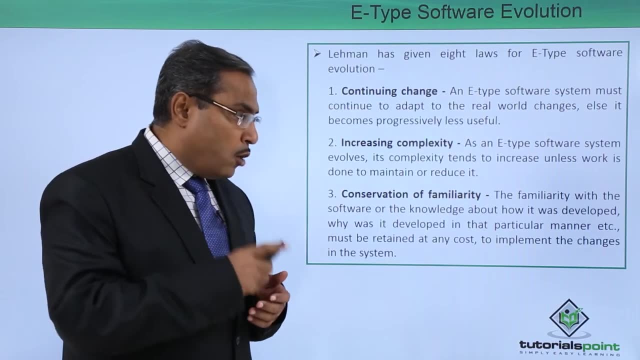 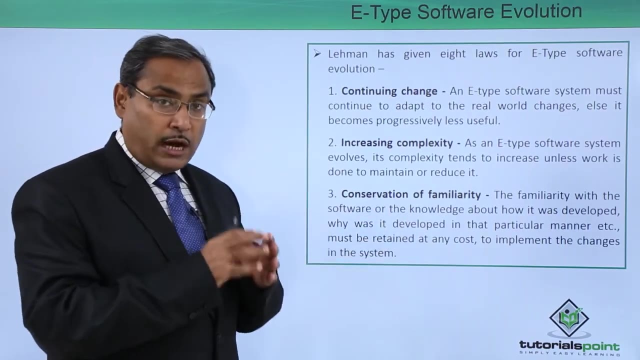 Next one is a conservation of familiarity. So what is the conservation of familiarity? The familiarity with the software, or the knowledge about how it was developed and why was it developed in that particular manner, etcetera. So they are to be preserved and conserved, must be retained at any cost to implement. 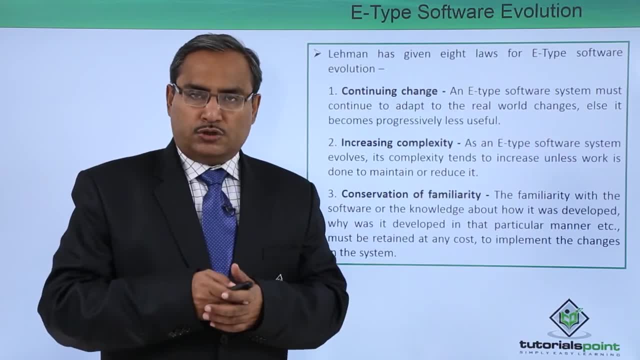 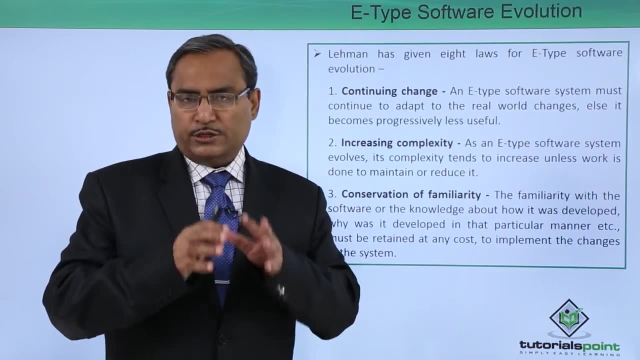 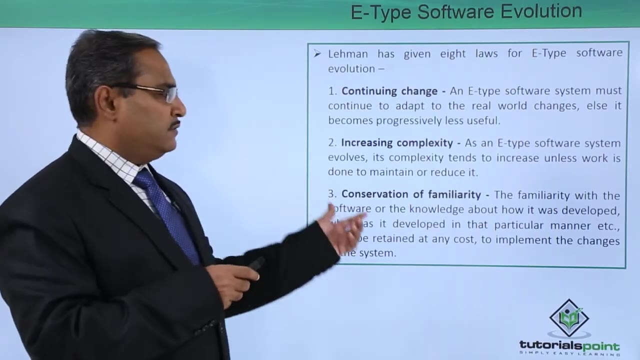 the changes in the software in the coming days. So all why this particular software has got developed in this way and how it has got developed in this way, all this knowledge must be kept, must be stored, so that this conservation will be required, this conservation. 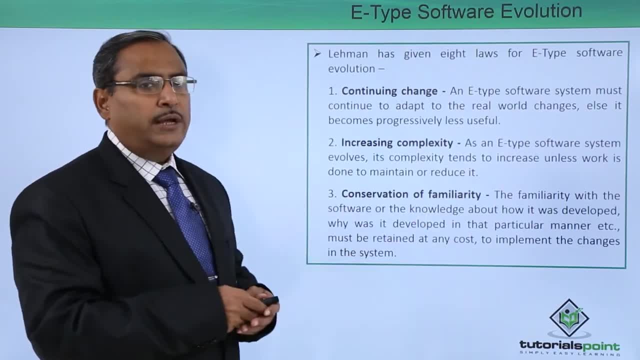 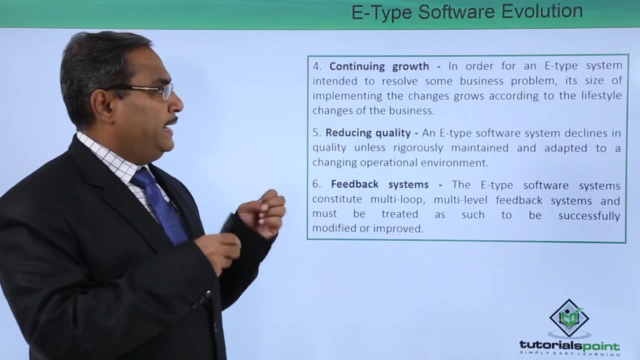 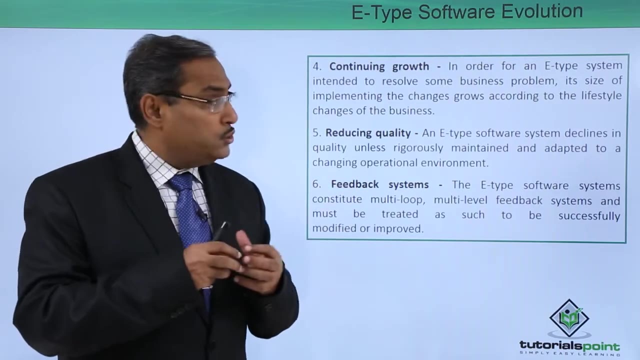 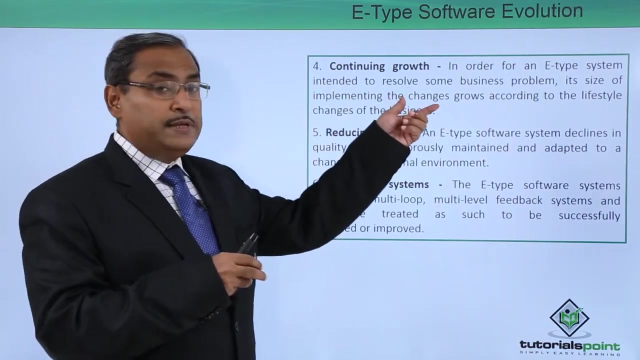 of familiarity will be required in the coming days to execute any kind of change. request: Continuing growth In order for an E-type system intended to resolve some business problems. its size of implementing the change grows according to the lifestyle change of the business. So the intended to resolve some business problems, So now you. 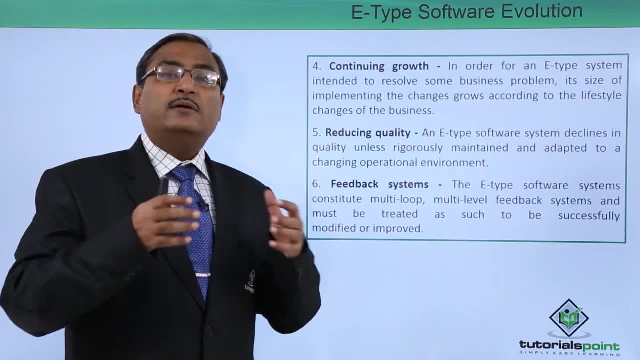 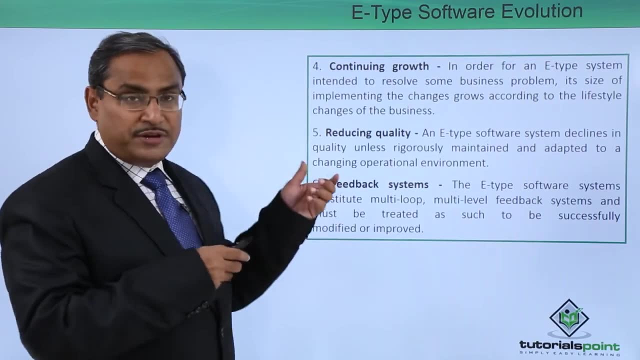 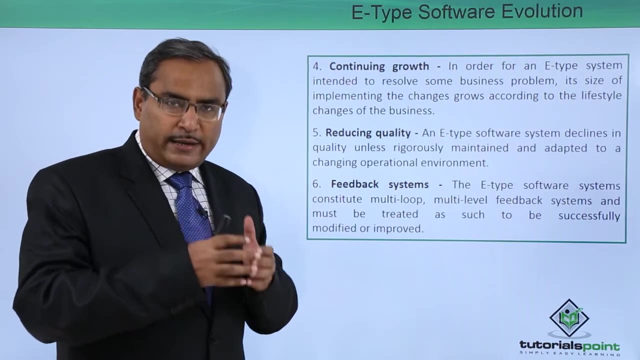 see its business, the lifestyle, the new wing may get introduced in the existing business. So as a result of that, whenever a particular software is going to implement those changes, the volume of that implementation of change will be directly proportional to the lifestyle.